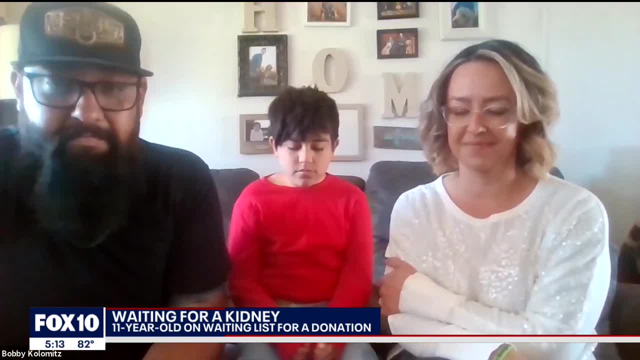 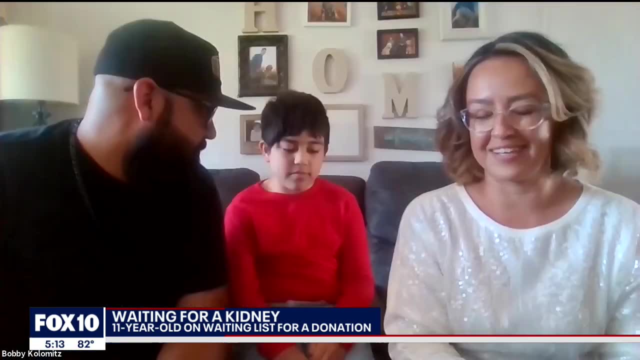 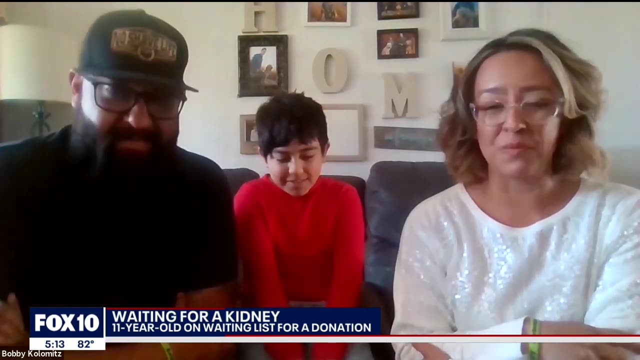 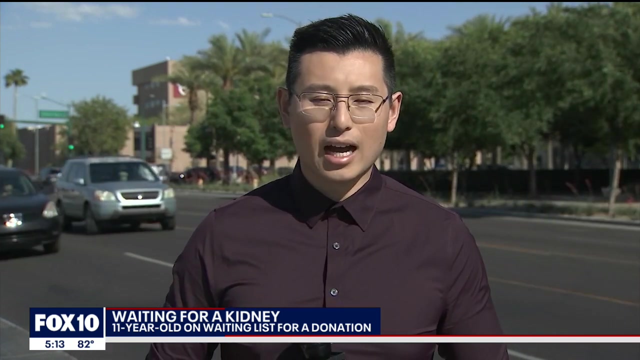 see if they can be living kidney donors. Our community is the best. there is No match yet, but hope is still very much alive that someone can save Tristan. I don't think there's words to express the gratitude we have for that to be able to- sorry, try to give him a little bit more normalcy to his childhood. If you want to register as a donor, just head to DonateLifeAZorg In Phoenix. Justin Lum Fox 10 News. 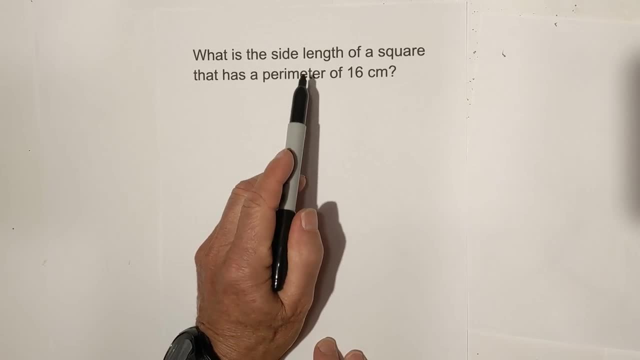 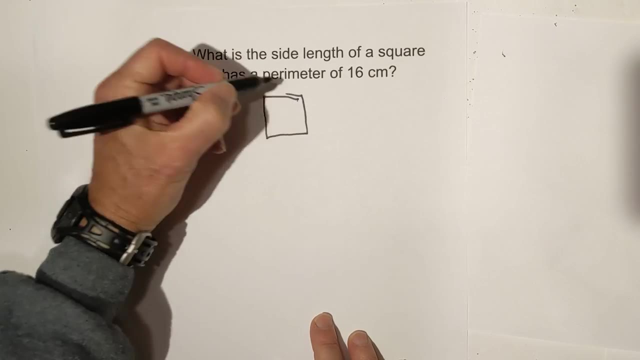 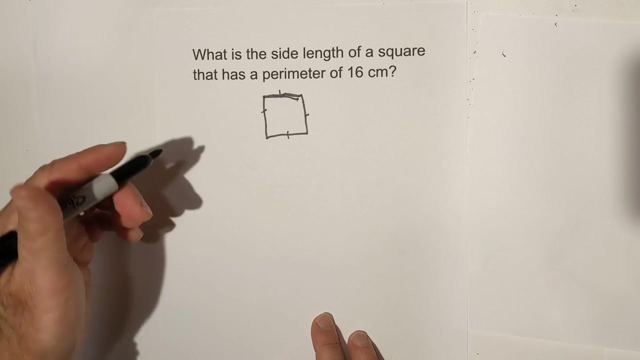 Welcome to MooMooMath and Science. In this video, let's find the side length of a square, given perimeter, And what's unique about a square is that- oops, that's a very poor square. All four sides are the same. They're equal. So what we can do is we can go: 4x equals the perimeter. 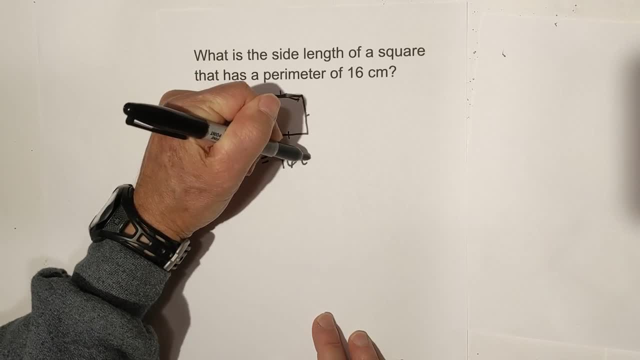 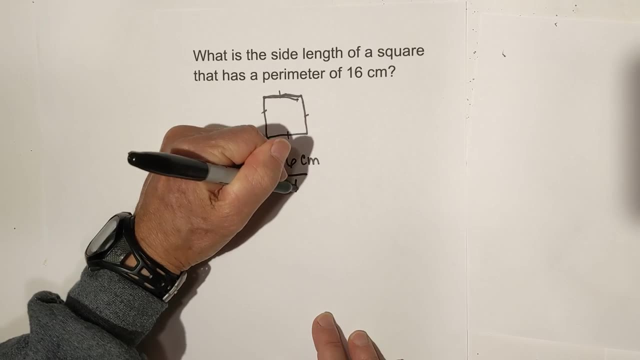 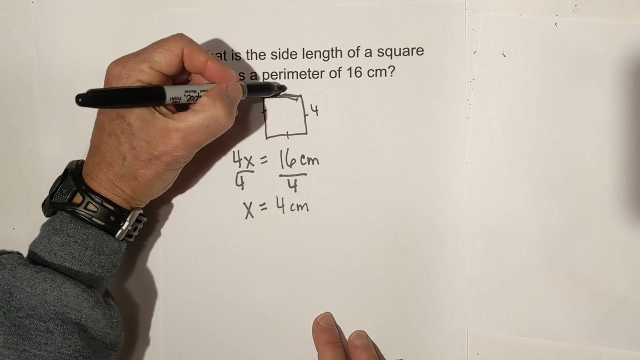 and the perimeter in this particular example is 16 centimeters. So then all we do is we get x by itself by dividing by 4.. So x is equal to 4 centimeters, And so this is 4,, 4,, 4, and 4,. 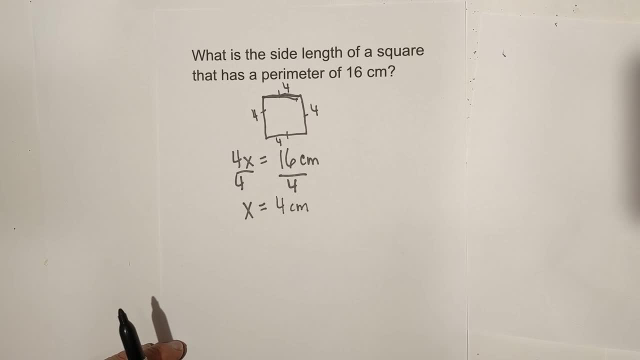 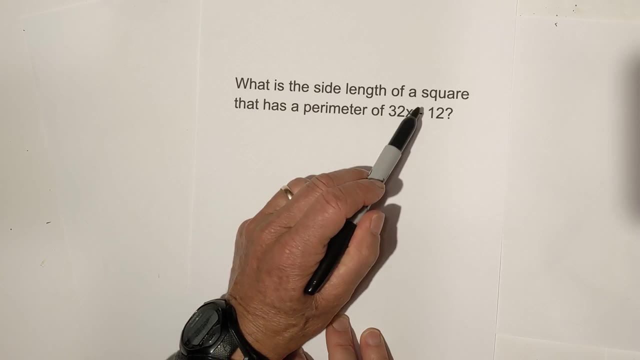 and that adds up to 16.. Okay, let's look at another example. In this example we're given some variables, etc. So we have: what is the side length of a square that has a perimeter of 32x minus 12?? So again, 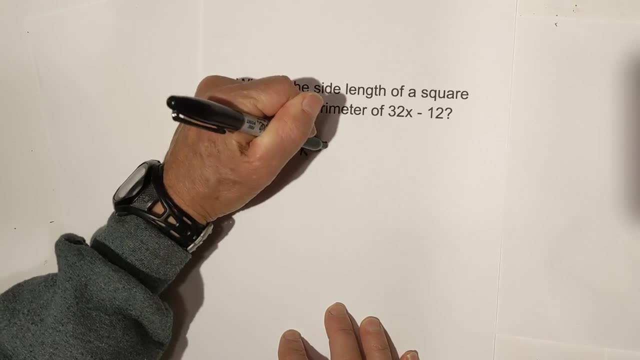 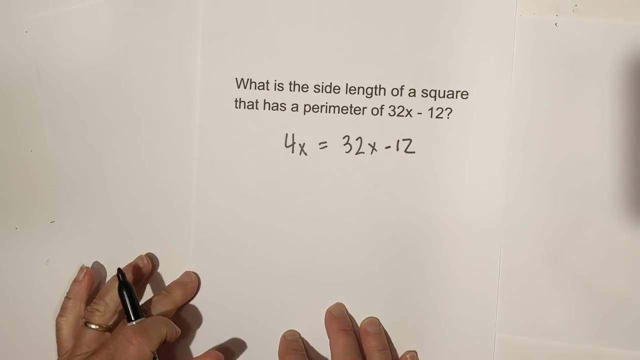 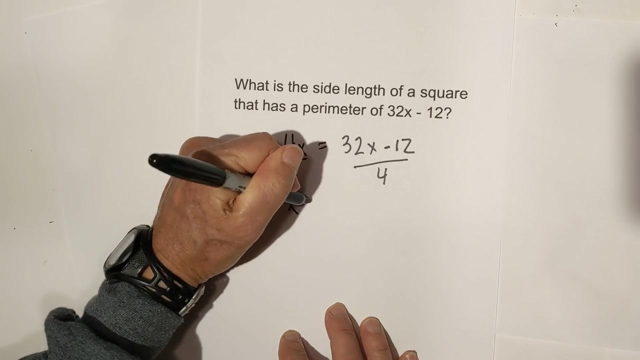 what we will do is we will just set up 4x, which is 4 times each side, and it's going to equal 32x minus 12.. Then all we do is get x by itself by dividing by 4.. So x is equal to 4, goes into 32x. 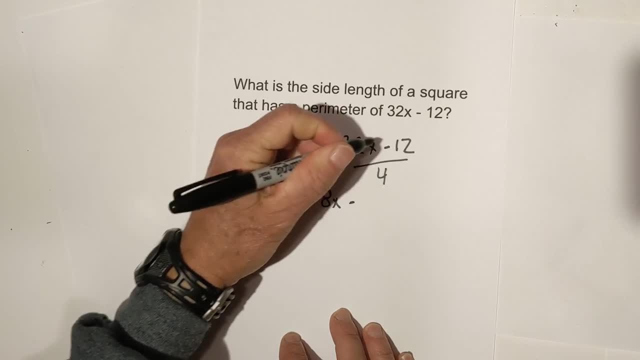 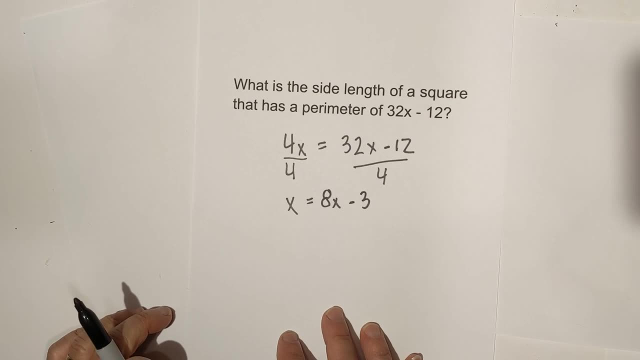 8 times 8x minus and 4 goes into 12 three times. So there we go. x would equal 8x minus 3.. I hope that was helpful. Thanks for watching and remember: kindness multiplies kindness, Be kind.